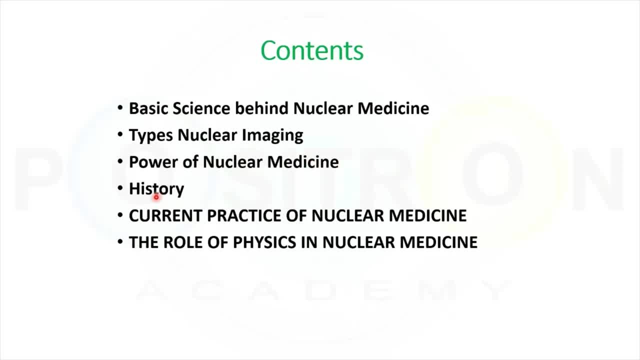 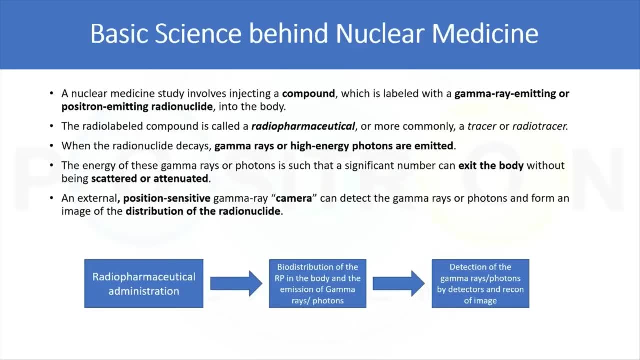 and with due time we'll talk about history and the current practice of nuclear medicine and the role of physics in nuclear medicine. let us discuss the basic science behind nuclear medicine. so a nuclear medicine study involves injecting a compound and this compound is labeled with a radionuclide and which decays by emitting gamma rays or 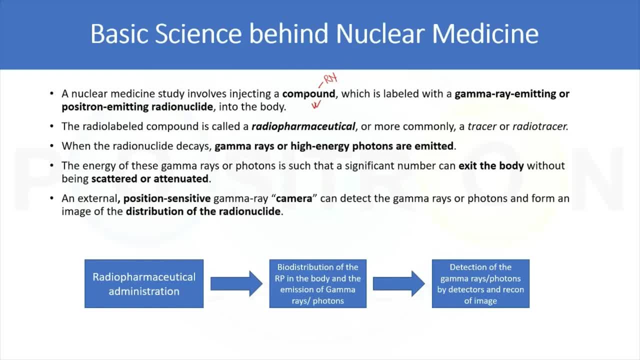 in the form of radio nucleotides and which decays by emitting gamma rays, or in the form of radio nucleotides and which decays by emitting gamma rays or positron into the body, and this compound, along with this radionuclide, is being called as a 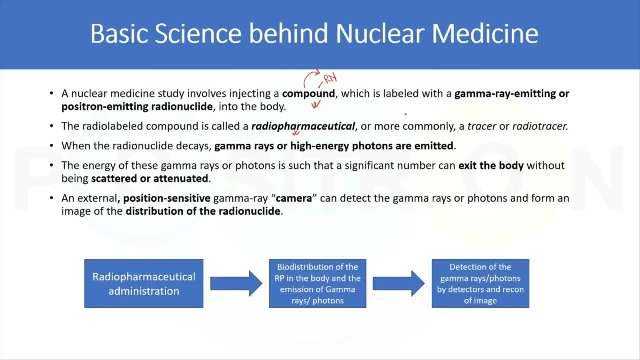 radiopharmaceutical, or more commonly as a tracer or a radio tracer. so when these radionuclide decays, gamma rays or high energy photons are emitted and these gamma rays have sufficient energy that it can leave the body in significant number without being scattered or attenuated and there is an external position sensitive gamma camera, 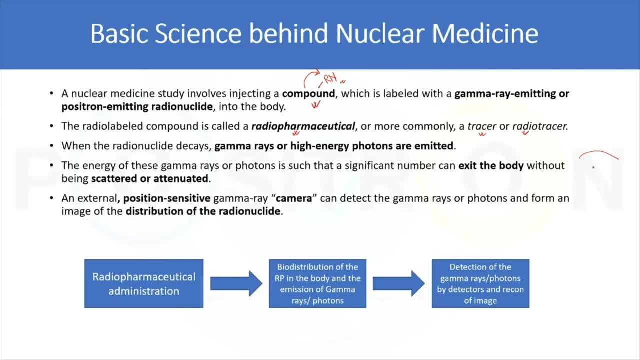 it can detect the gamma rays or the photons and can form the image of the distribution of the radionuclide. so in summary, we can sum out that how a nuclear medicine scan is being done. so it all starts with administration of the radiopharmaceutical, and this pharmaceutical is specific for a given. 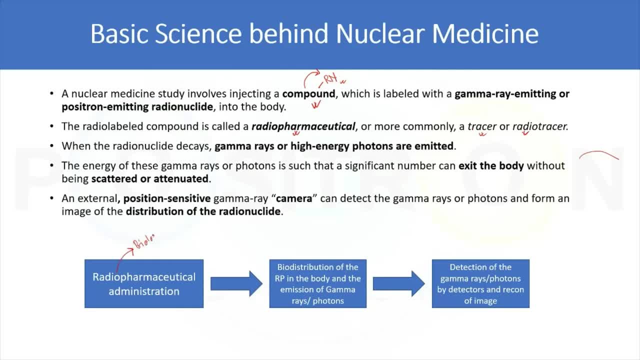 biological process, fine. so post administration of the radiopharmaceutical. so this pharmaceutical biodistributes in the patient's body and also lead to the emission of the gamma ray photons. fine. and the last step is detection of those gamma ray photons emitted by the radiopharmaceutical. 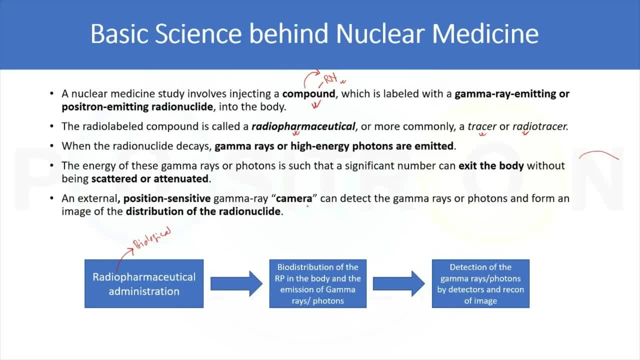 for reconstruction of the medical image, and that image tells us that the radiopharmaceutical is going to be used to detect the gamma ray photons. and that image tells us that the radiopharmaceutical is about the distribution about of the pharmaceutical inside the patient's 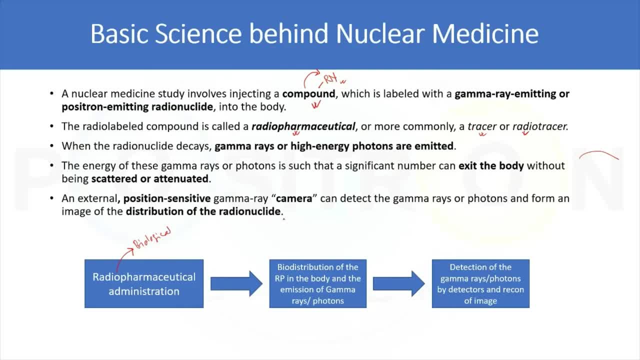 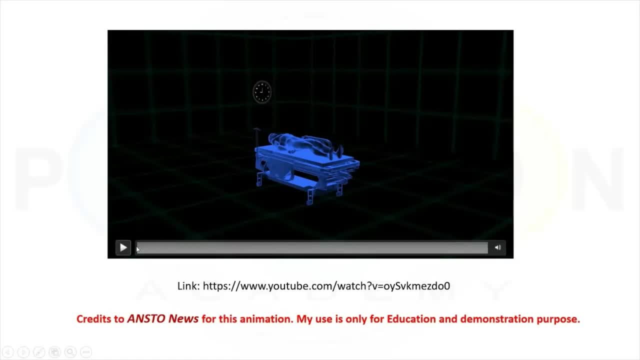 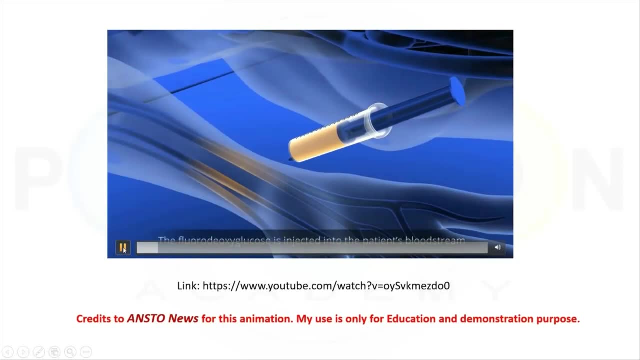 body, and this image has many prognostic as well as diagnostic information. so now, if we want to summarize how this nuclear medicine process has been governed, so it all starts by administration of a pharmaceutical. so that's the pharmaceutical over here, and the pharmaceutical that's being used in the video is datg, the fluorodeoxyglucose. 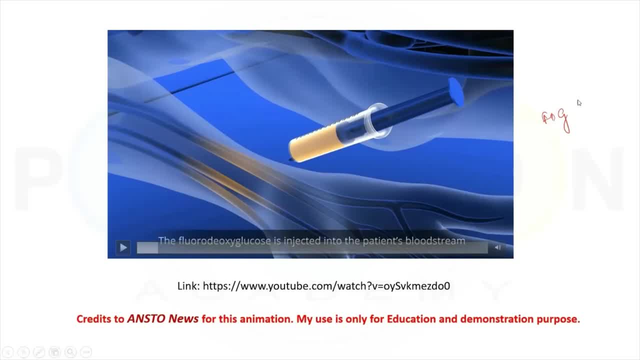 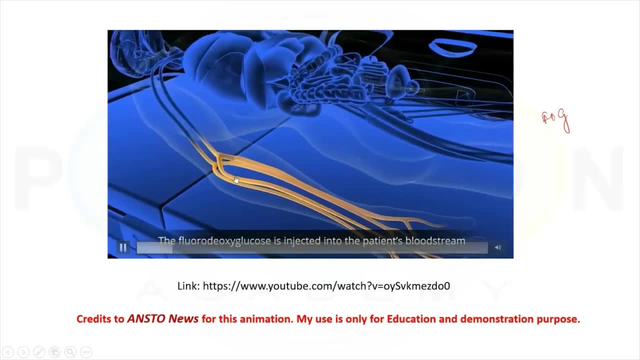 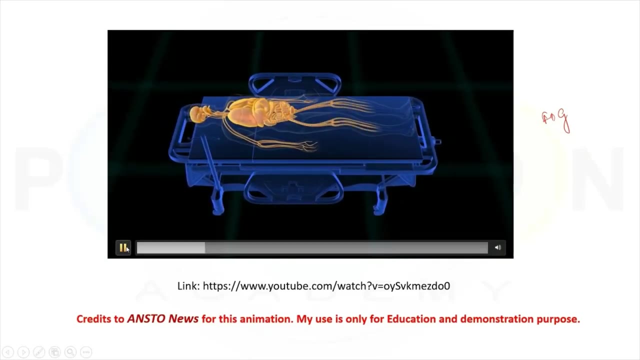 and that's an glucose analog. so once this glucose is being injected in the patient's bloodstream, so it goes and biodistributes in the patient's body. fine, and as we know, that's a glucose and we know our cells are quite dependent on glucose for deriving energy out of it through glycolysis and multiple other. 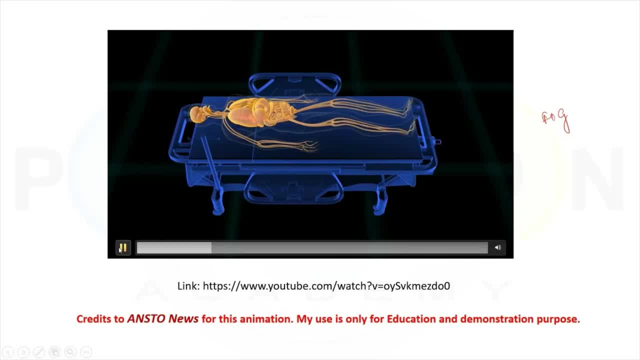 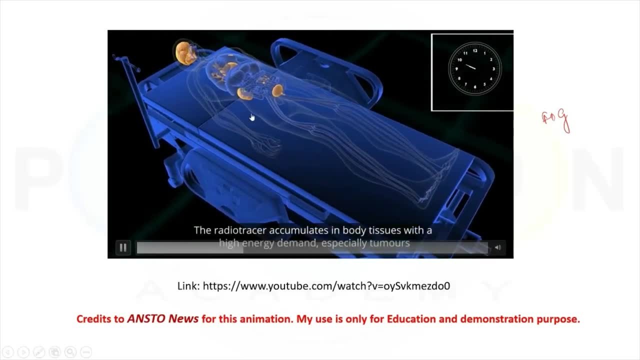 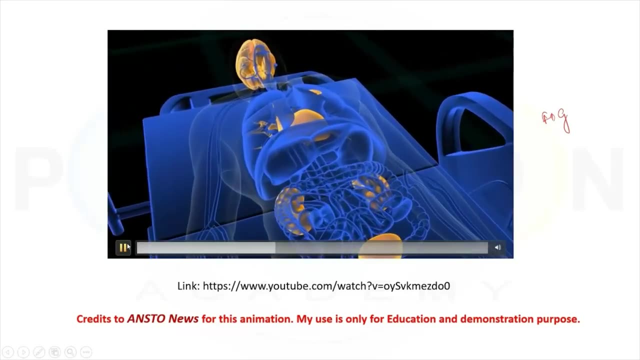 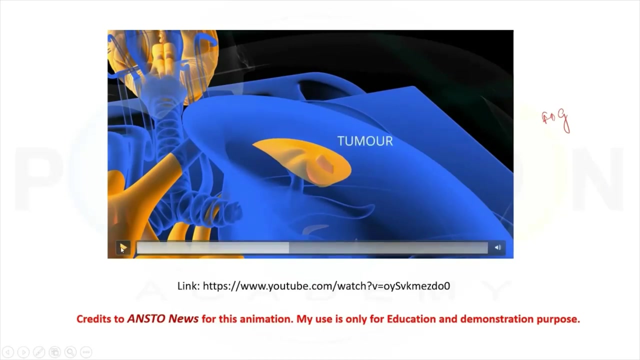 metabolic pathways. so we can see that glucose is taken up by our. our normal organs like brain has taken glucose at higher concentration. kidneys, blooders have taken glucose. but one thing that we can notice over here that the patient's lung has a small tumor and the tumor has also taken up glucose. why so? the answer. 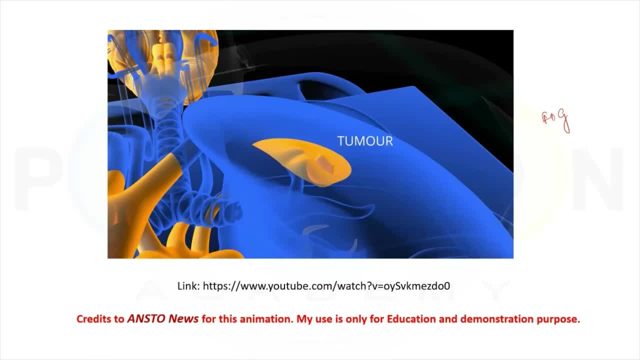 is that tumor are glycolytically more active. they have over expression of blood transplants voters and with this our Express load transporters. they have taken more glucose. so we can now see that tumor has taken more glucose then the surrounding normal tissue, normal cells, and that is being used as a 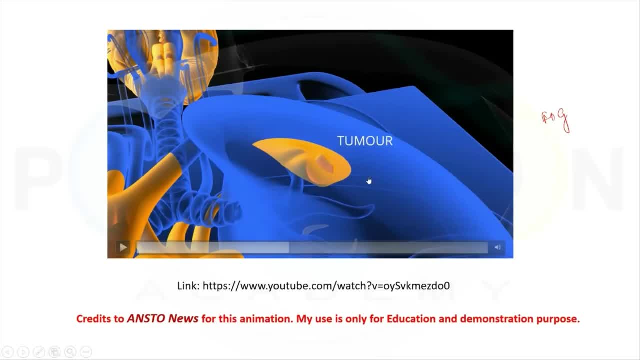 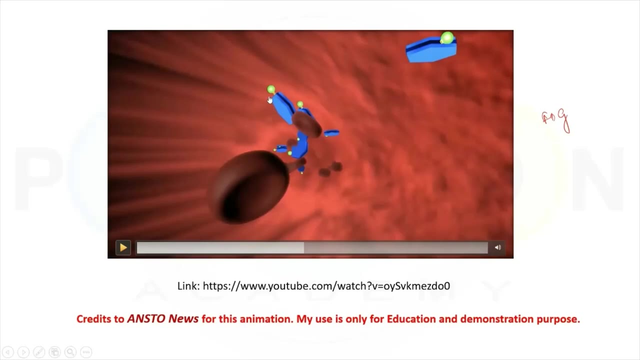 contrast between the uptick of the pharmaceutical by lesion, an optic by the normal cell. that's a huge contrast, difference between the two. fine, that's the initial scenario in which you can see, but that's our very ultimate end-". radiopharmaceutical, that's the glucose and that's the radionuclide, that is f18. 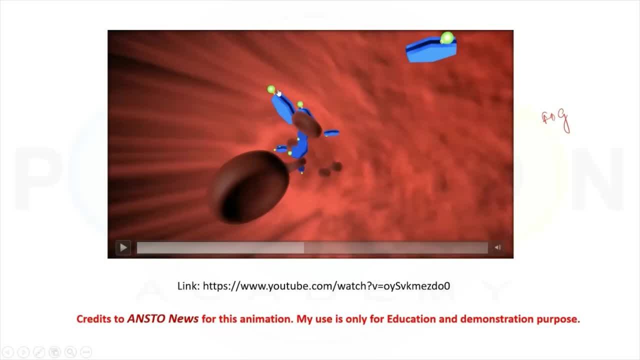 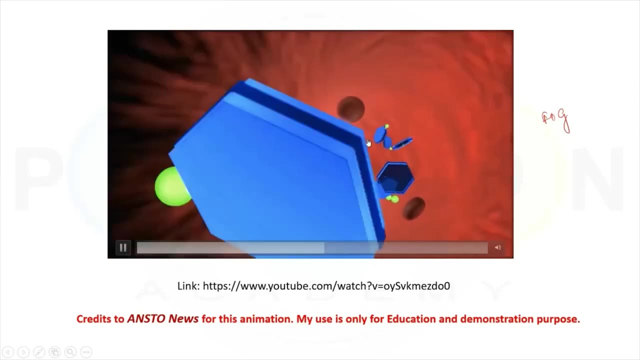 and, as I have told in my subsequent videos before, also that f18 is an positron emitter. fine. so what it does? it decays by emitting a positron and we can see that's our FDG in the bloodstream, and these FDG are taken more by the. 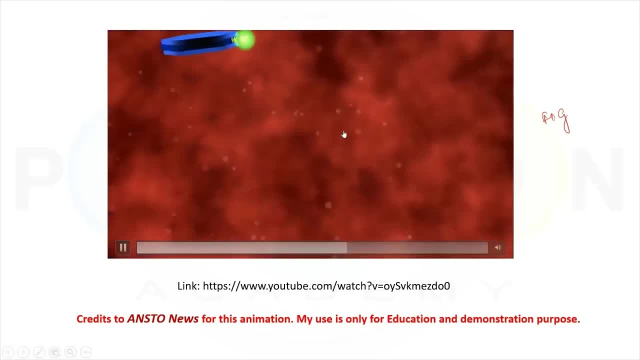 tumor cells. that's the f18 FDG over here, and it decays by emitting a positron and that's the positron over here. and this positron has a definite range in our normal, in our tissue, and what it does? it keep on annihilating. 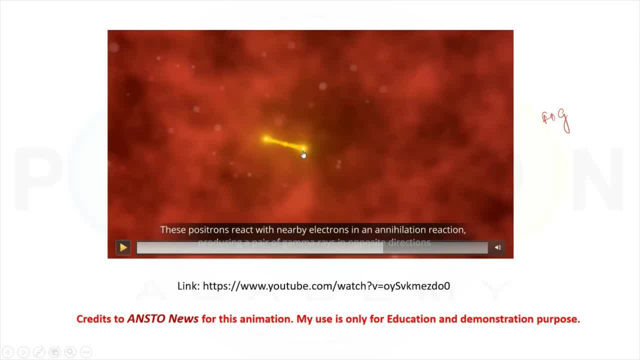 with an electron. so these, at this position, this positron and the electron has annihilated, has combined and resulting the production of two high energy gamma ray photons having energy equals to 511 kilo electron volt. so these are the two high energy gamma ray photons emitted by these positron, positron annihilation. 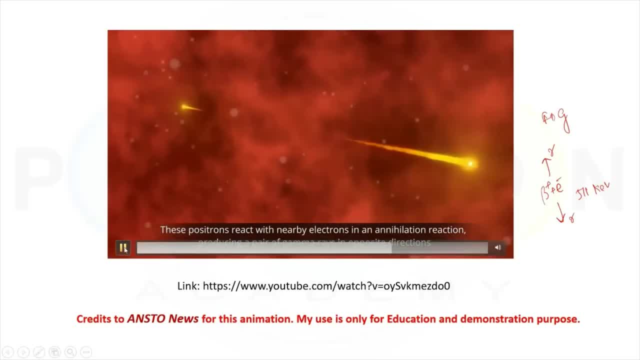 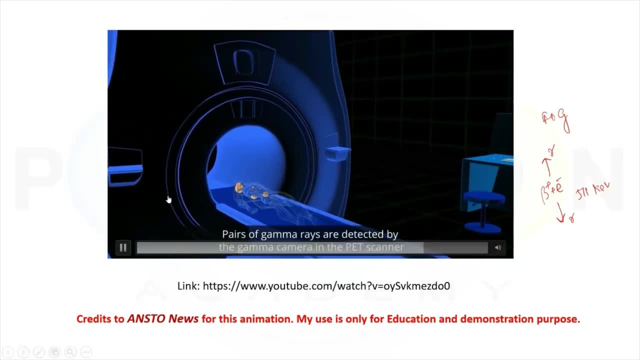 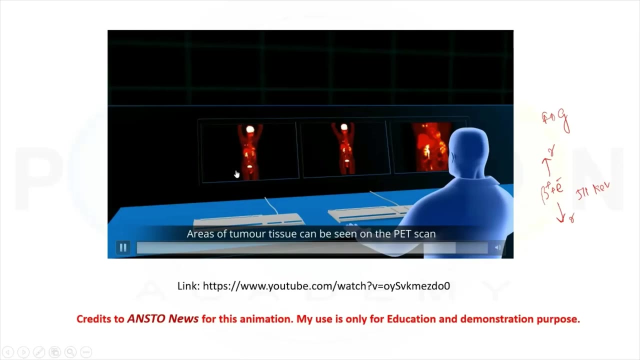 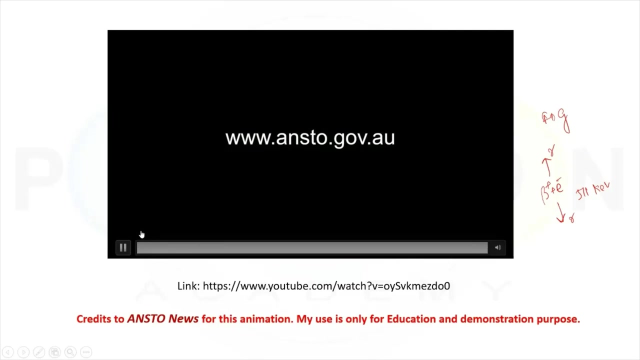 process and these gamma ray photons have been detected by the position sensitive PET cameras and are being used for reconstruction of the medical image. and that's the medical image over here and that's tell us more about how these radiopharmaceutical has has distributed inside the patient's body. so now we can see how a nuclear 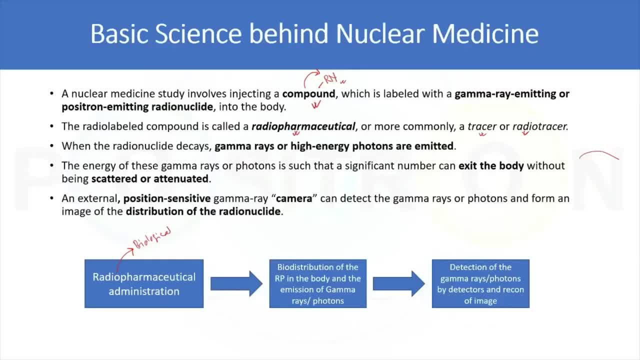 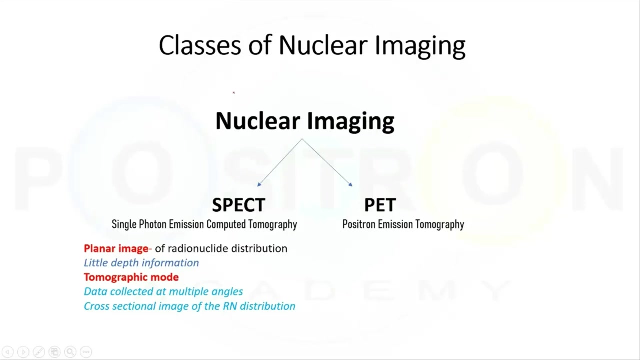 medicine study goes through. first step is obviously pharmaceutical administration, followed by bio distribution of the pharmaceutical in the body and also the emission of the gamma ray photons and finally detection of this gamma rays photon by detectors and reconstruction of the medical image. fine, so now the next is on the classification of nuclear imaging, and we can broadly 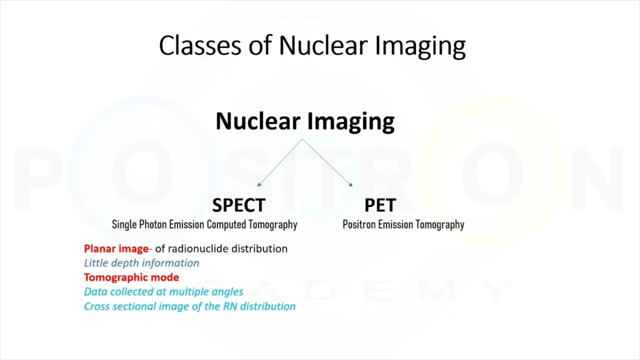 classify nuclear damaging Intwo main subdivisions. it can be either and packed imaging or pet imaging. so what is packed imaging? forty experiments: single photon emission, computer tomography. but is why we call is single photon, because the radio declares that are being used teen expect the case. by emitting a single formic atom, you layer trapped by emitting a single photon smoke. hICESF clues. thanks for watching. 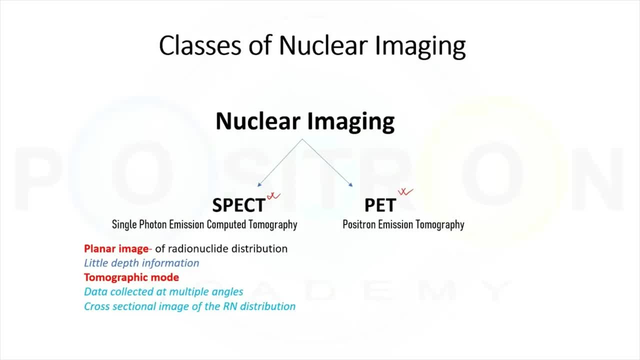 so understanding is to pay that you neglected. been used in is a pre tuned to to protect the case by emitting a single photon emission, computer tomography first, and power heartthen zero sing electron emitting bluetooth Empressッab hint from the top of the heta to give you a good idea about atom when you detect. 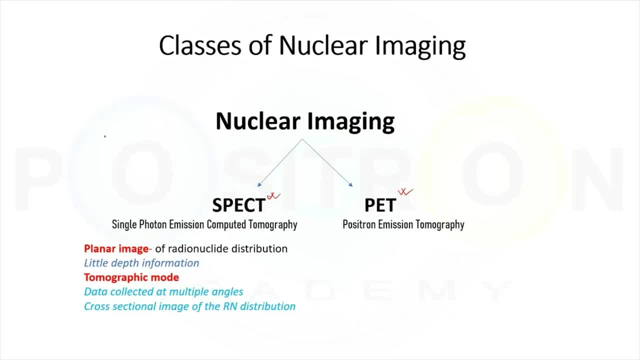 emitting a single photon part disintegration example: the most commonly used radionuclide inspect is 99m technetium- technetium at a stable state. so it decays to technetium stable by emitting a gamma ray photon. so how many gamma are being released? one gamma, that's why I call a single photon. now 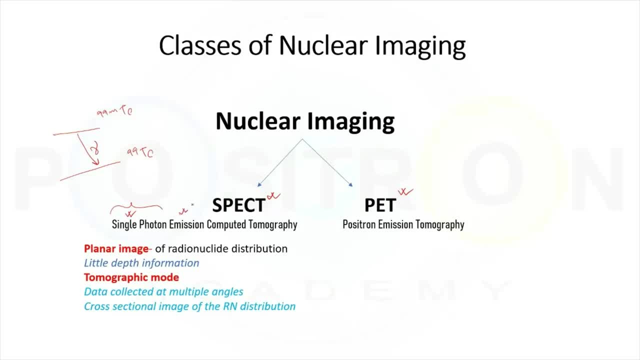 why we call as emission: emission because the patient's body emits the radiation. that's why we call is emission. and why we call is computer tomography, because the reconstruction process employed inspect is similar for by, for of the reconstruction followed in CT scan. that's why we call is computer. 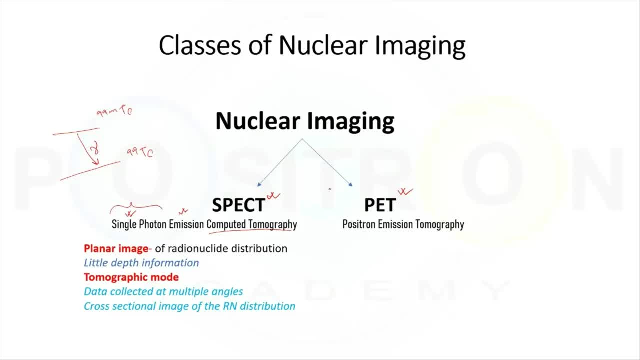 tomography. and now I guess you are quite familiar why we call a single photon emission computer tomography? because a single photon is being released, emission because patient's body emits radiation, and of and why city? because the process, reconstruction, employed, inspect, is taken from the reconstruction from CT. 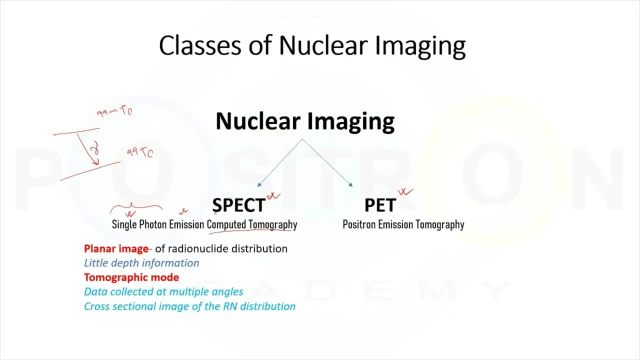 scan. that's why computer tomography and this fact imaging can generate both planar image as well as tomographic image. so in planar image it has a demerit that it cannot provide you depth information and it provides you little depth information. but virus for tomographic image it provides us depth. 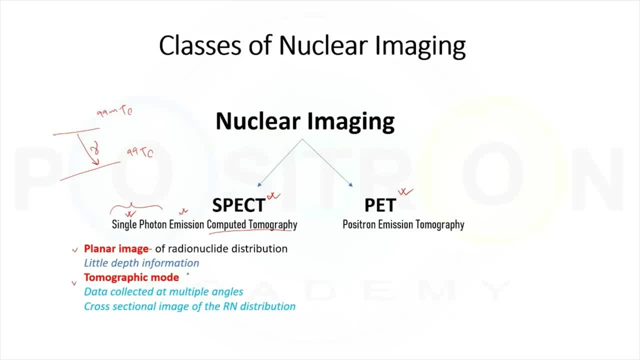 information also and for the same datas are collected at angles and and cross-section of image of the rate of the radionuclide distribution is being obtained, and regarding a PET imaging. the radionuclide used in PET is decays by means of emitting a positron. 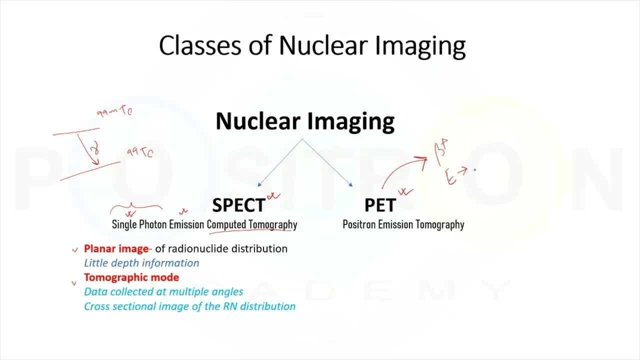 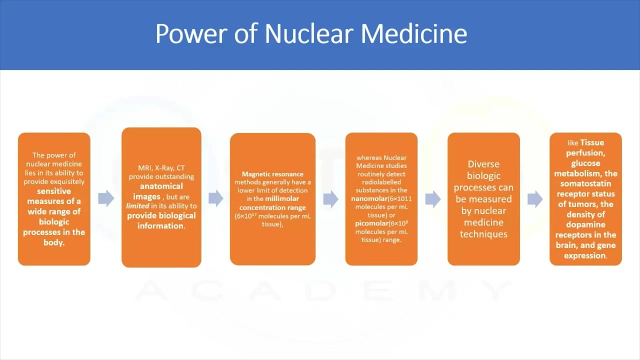 and why? emission because patients body emits radiation, and tomography because image that have been formed are the slice by slice, image are being generated. that's why you call it tomographic images. and regarding how it goes on, I have explained in the previous video how PET imaging goes through. next topic of discussion is on the power of nuclear medicine. so what's? 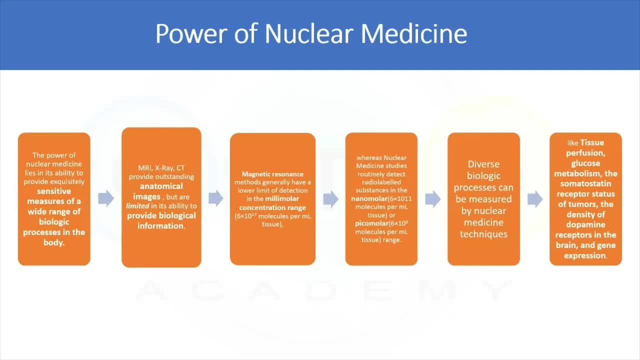 the advantage of going through a nuclear medicine study? what's the added advantage of the same? so the main power of nuclear medicine lies in its ability to provide sensitive measures of a wide range of biological processes in the body, and it can provide information even at the molecular level. so if we compare nuclear 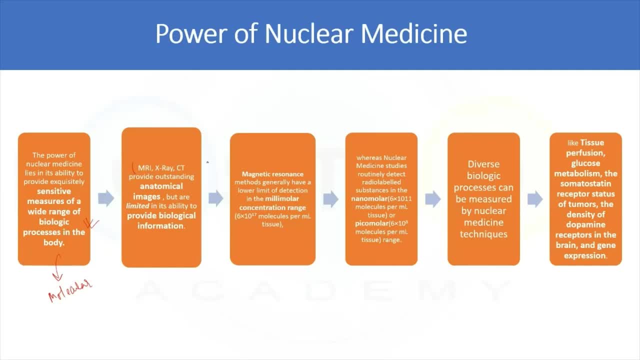 medicine study with other studies like MRI based study, X3 based study or CT based study. they provide information at the anatomical level, but they cannot provide information at the molecular level. and even nuclear medicine studies have very high sensitivity, even at the nanomolar range or at picomolar range of the radio's level. substance concentration. 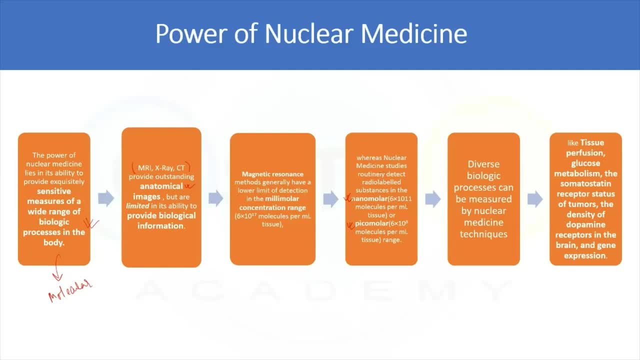 and by means of nuclear medicine you can study diverse biological process, like you can study tissue perfusion, glucose metabolism, somatostatin receptor expression and many more things. so you can study events, what are going on at the molecular level. fine, not at anatomical scale, so that that will. 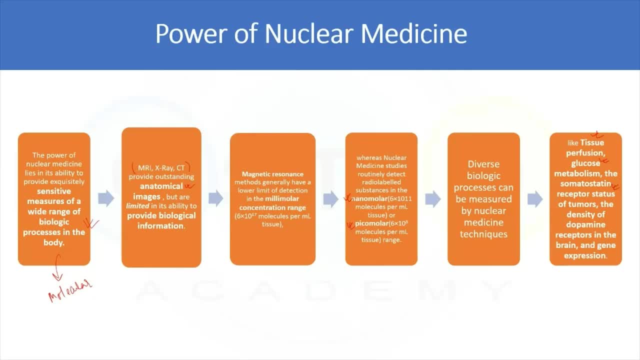 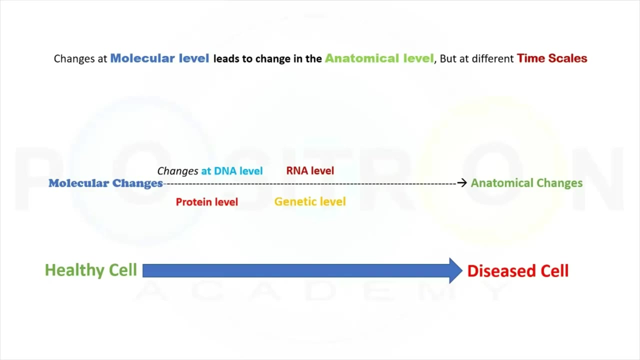 tell more about what's going at the cellular level or at the genetic level. it has the ability to tell you even at that scale. so the next question is why knowing biological phenomena at the molecular level is important. so the answer is: for example, when a healthy cell get transformed to a diseased cell, so in a healthy 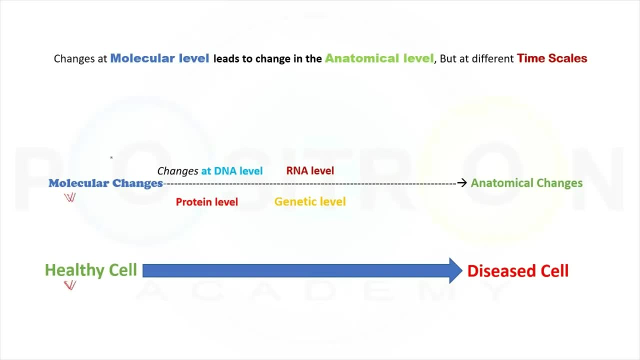 cell, there occur some of the molecular changes, and these molecular changes can be at the DNA level, can be at the RNA level, can be at the genetic level or at the protein level or at any other levels. and because of these changes at these level, this molecular level or other things or other things, 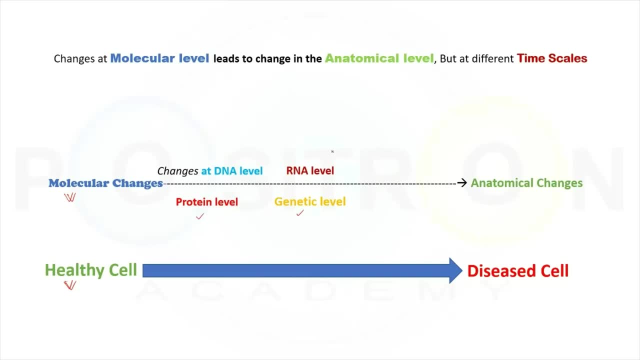 or a single cell level. there occurs changes at them at the anatomical level also, so these changes occur at later time points. and these changes occurs at at earlier time points, maybe even months, years before the disease can be seen. fine, so by means of molecular imaging if we can sense out the change. 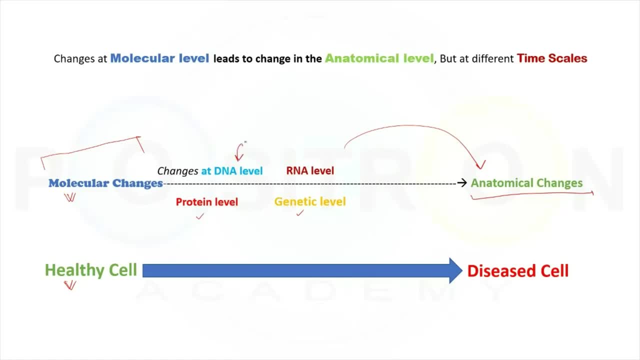 at the molecular level, we can diagnose disease at an earlier stage, and that's the advantage of nuclear imaging, that it can detect changes at earlier stage at which anatomical changes has not yet occurred. fine, so changes at molecular level lead to change in the anatomical level, but at different time. 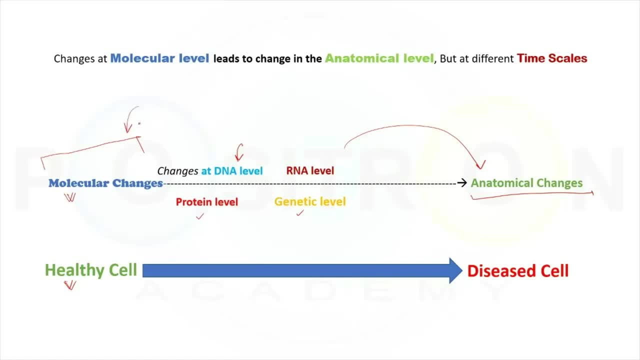 scale. the tea is that this molecular changes occur very early, like changes in DNA level, changes in protein expression. this occurs very early and because of this accumulation of these changes over time it lead to a significant anatomical change. and then we got to know that we have a disease, so by means of nuclear medicine. 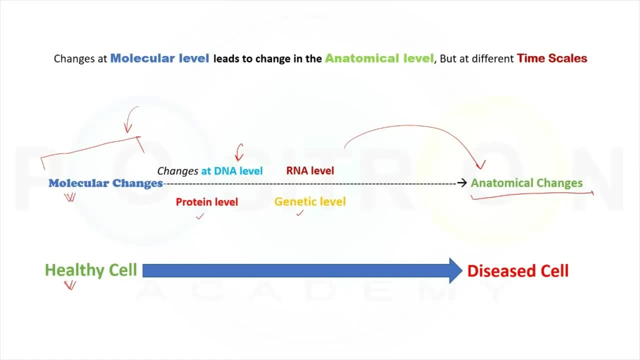 if I can predict that I am going to have to have this disease, then treating disease becomes much more easier. and that's the advantage of nuclear medicine, that it can detect those molecular changes at the molecular level and can prevent disease or can treat disease at an earlier stage. 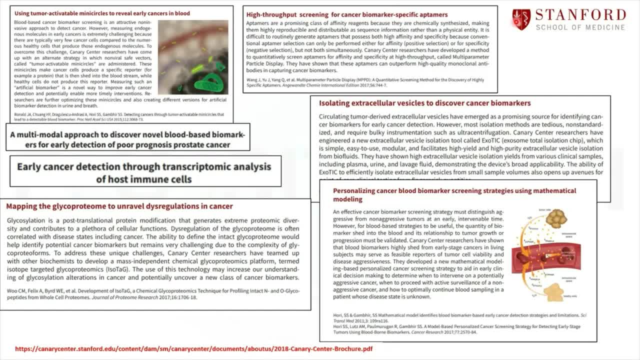 of time. so these are the series of research works done by people at Stanford School of Medicine, and their main motto was to to discover those early changing biomarkers. and if you can detect those early changing biomarkers, then then disease treatment- this is detection- becomes much more. 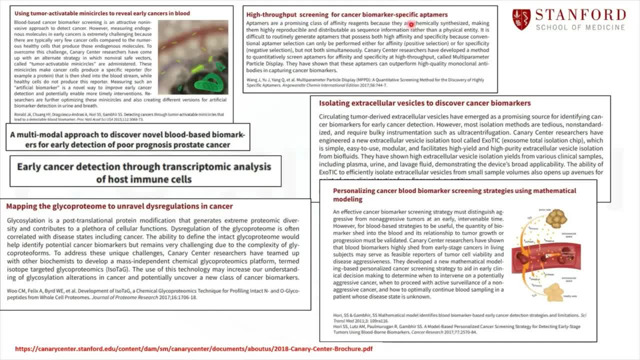 easier and also the patient's life also keep on increasing. so by using this group of research, uh, the main effort was to find out the early changing biomarkers. so by using a tumor activity- my mini circles- they can unravel early change, early cancers in blood. and there are different approaches which 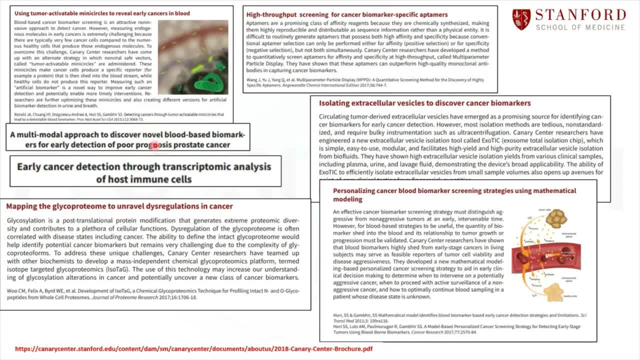 are being used for the detection or discovery of the novel blood-based biomarkers for early detection of poor prognosis prostate cancer, and they are also trying to map the glycoprotein to unraveled dysregulation and cancer and so on and so forth. so these are series of researches done. 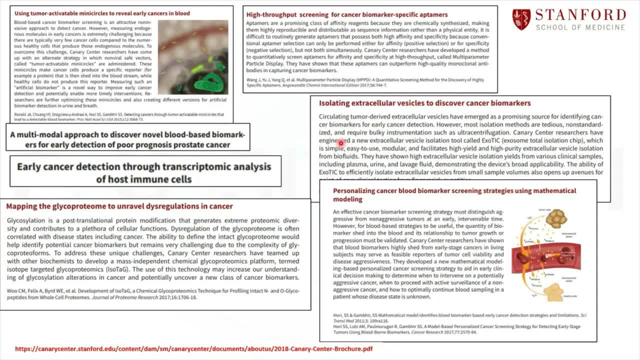 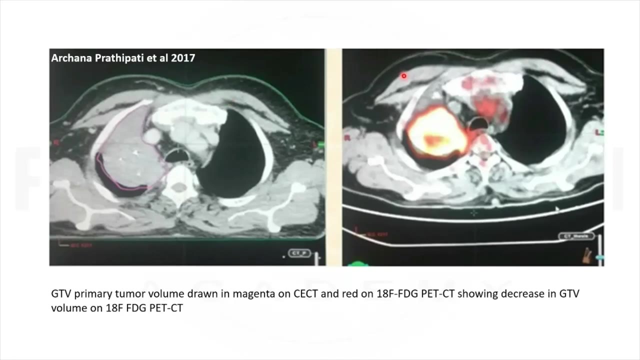 at Stanford School of Medicine with an aim at finding out those early changing biomarkers. so if you can, if you can image those early changing biomarkers, or if you can detect those early changing biomarkers, then the disease detection, disease diagnosis and disease treatment becomes much more easier. so that's an uh CT image and there's an pet city image of the same patient. 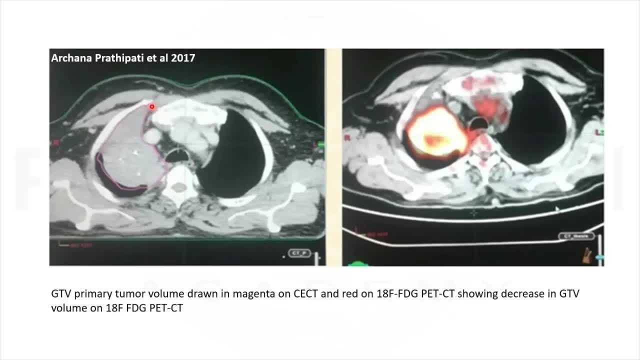 and what we can see over here, that's a. there's a tumor in the patient's right lung. fine, so that's the only thing that we can observe in this anatomical imaging: that we can see the still long lesion over here. but we cannot tell looking at this image. 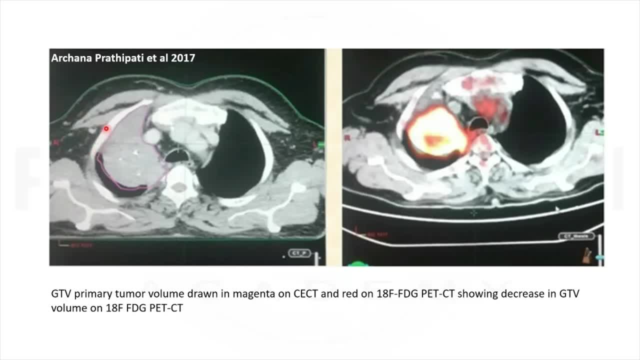 how much receptor are they expressed on the tumor surface? or what about the metabolic rate of this particular lesion? so, but by means of f-18 FBG pet city scan, we can now tell the volume of tumor that is glycolytic, glycolytically active. so now, by means of nuclear medicine, we are revealing. 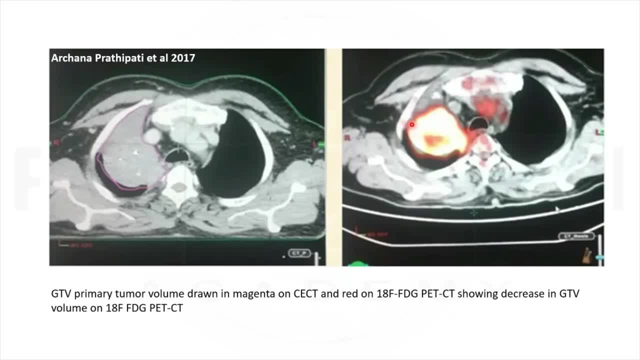 information at the molecular scale also because this group of this volume of the, this volume of this tumor is glycolytically more active. so what it means? they have higher expression of the glute rotors. so by means of nuclear medicine we are revealing something more than this anatomical 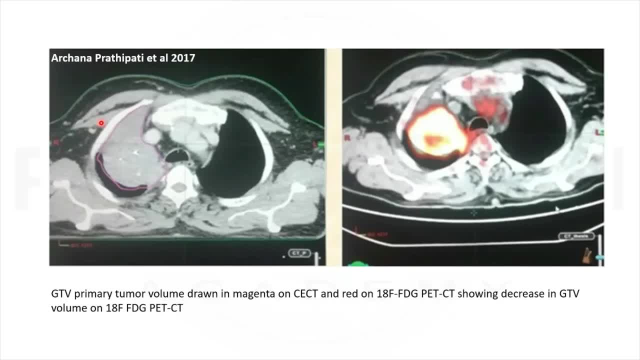 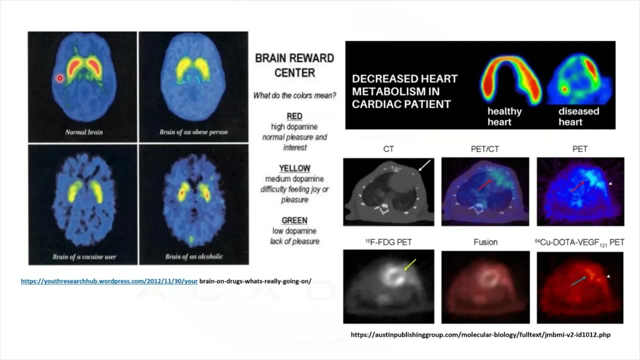 imaging. we're now telling you about the glycolytic rate, about receptor expression and many more things, and that's the advantage of nuclear medicine, that it can tell you more about what's going on in the molecular level. and that's about some of the normal brain scans we can see. in a normal brain there is.